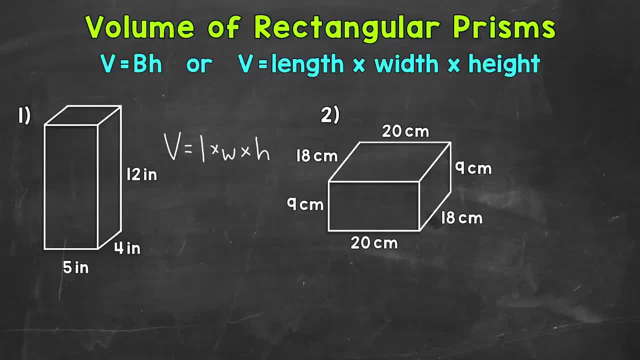 Width and height. Now, I never get too held up on which dimension is the length of our base and which is the width of our base. As long as we are using the 5 inches and the 4 inches, we're going to get the correct area of that base. 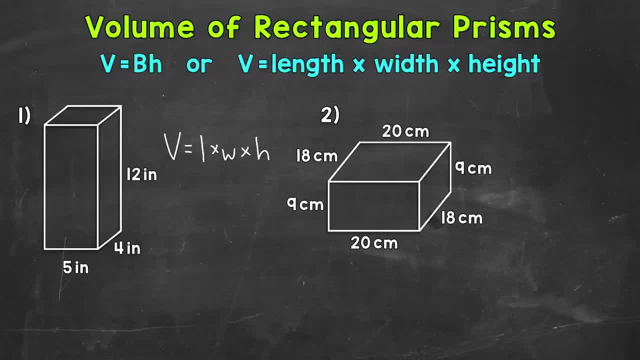 and therefore the correct volume of the rectangular prism. I'm going to use the longer dimension, 5,, for our length, and the shorter dimension for our length. I'm going to use the longer dimension, 4,, for our width, in order to keep things consistent. 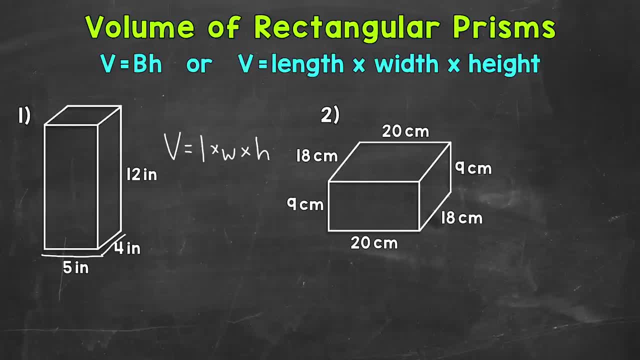 So that's a common way of doing things when it comes to length and width, Using the longer dimension for length and then the shorter for the width. But again, don't get too held up on this, because 5 times 4 equals 20, and 4 times 5 equals 20.. 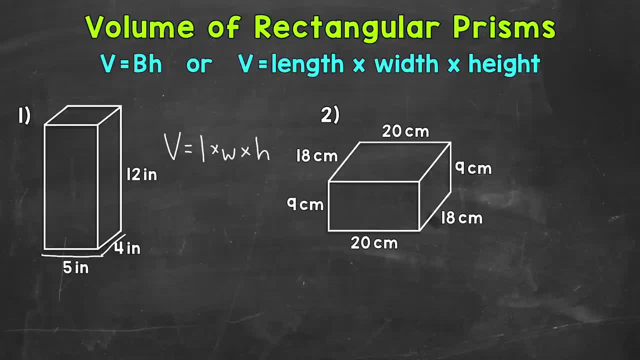 So either way, you're going to get the correct area of the base, which is going to be 20 square inches. So let's plug in our length. So let's plug in the length and width here, So the length of 5 times the width, of 4 times our height, of 12 here. 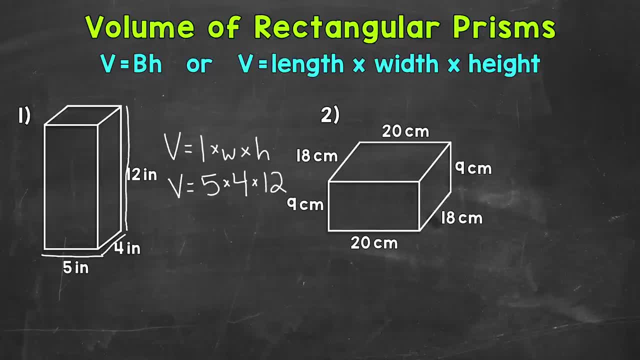 So 5 times 4 times 12 is going to give us the volume of this rectangular prism. So let's do one step at a time here. 5 times 4 gives us 20.. That's the area of our base, And then multiply it by the height of 12.. 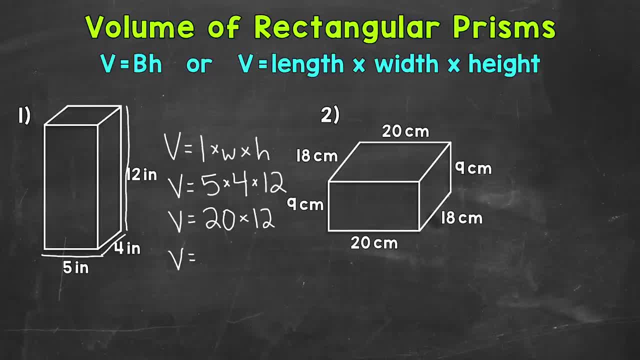 So 20 times 12, that's going to give us 240.. Now we need to remember our unit of measure. here Our answer represents how many cubic units fill our rectangular prism. So for number 1, we have cubic inches, So we can put inches and then cubed. 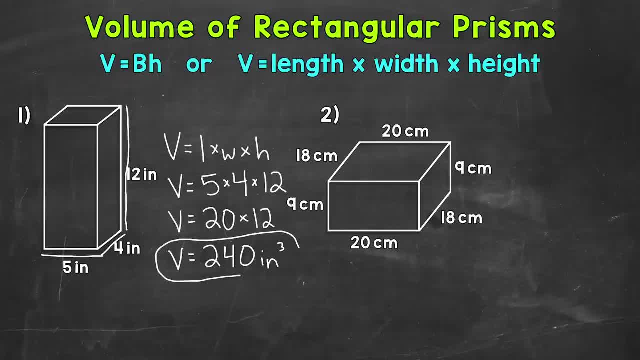 So 240 cubic inches as far as the volume Of number 1.. Let's move on to number 2, where we have another rectangular prism, But for this one we have more sides that are labeled, So we really need to know what we're looking for here as far as length times, width times, height. 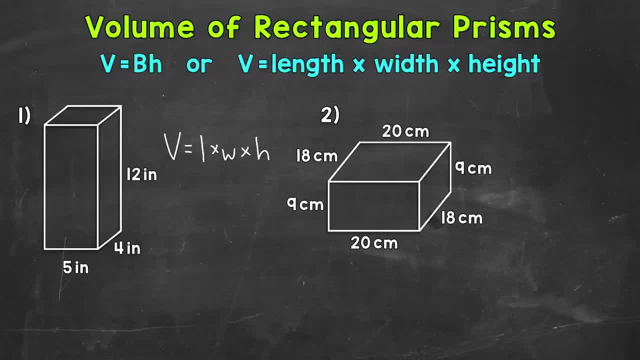 and therefore the correct volume of the rectangular prism. I'm going to use the longer dimension, 5,, for our length, and the shorter dimension for our length. I'm going to use the longer dimension, 4,, for our width, in order to keep things consistent. 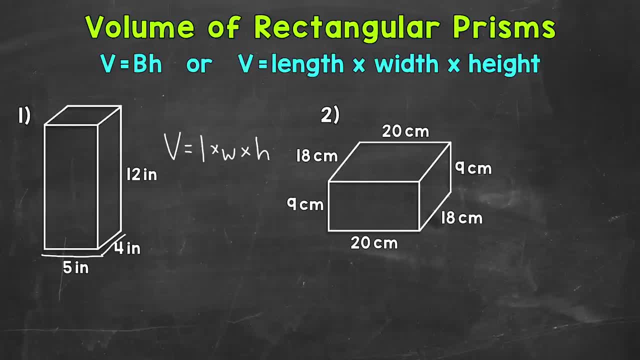 So that's a common way of doing things when it comes to length and width, Using the longer dimension for length and then the shorter for the width. But again, don't get too held up on this, because 5 times 4 equals 20, and 4 times 5 equals 20.. 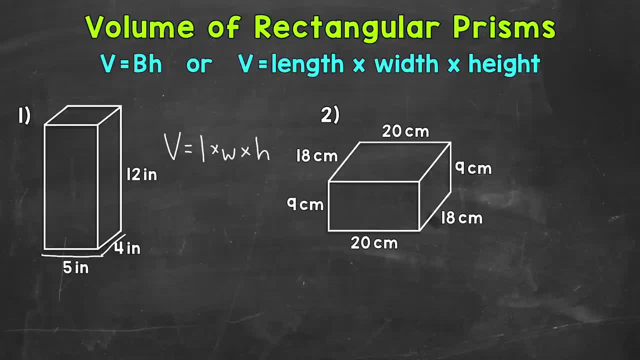 So either way, you're going to get the correct area of the base, which is going to be 20 square inches. So let's plug in our length. So let's plug in the length and width here, So the length of 5 times the width, of 4 times our height, of 12 here. 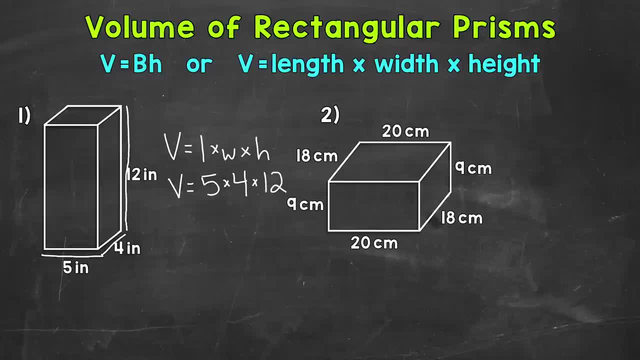 So 5 times 4 times 12 is going to give us the volume of this rectangular prism. So let's do one step at a time here. 5 times 4 gives us 20.. That's the area of our base, And then multiply it by the height of 12.. 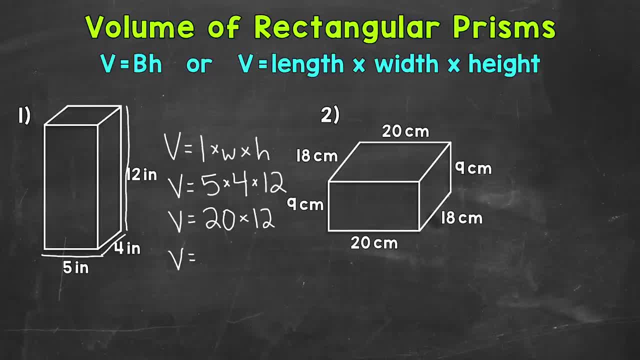 So 20 times 12, that's going to give us 240.. Now we need to remember our unit of measure. here Our answer represents how many cubic units fill our rectangular prism. So for number 1, we have cubic inches, So we can put inches and then cubed. 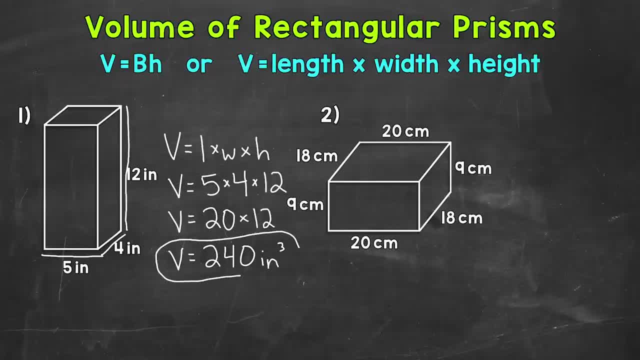 So 240 cubic inches as far as the volume Of number 1.. Let's move on to number 2, where we have another rectangular prism, But for this one we have more sides that are labeled, So we really need to know what we're looking for here as far as length times, width times, height. 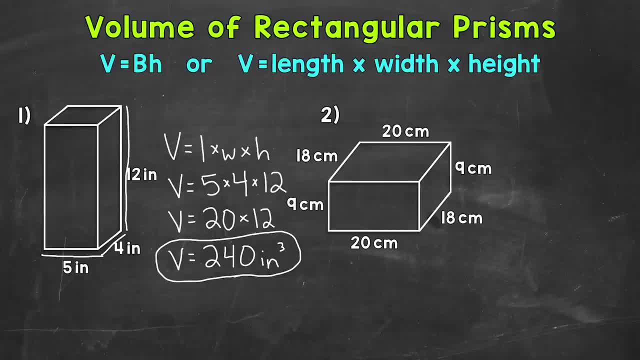 Don't just multiply all of the numbers that you are given. We need to be very careful here. So let's write out our formula: Volume equals length times width times height. So now we need to know what we're looking for. We need to plug in the length and width of our base.